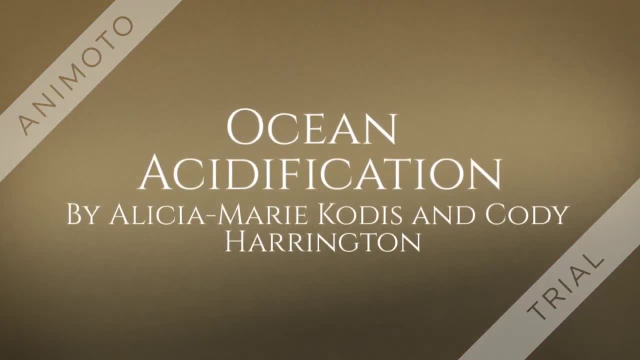 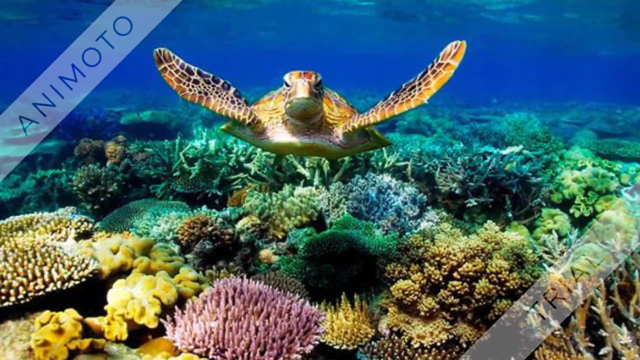 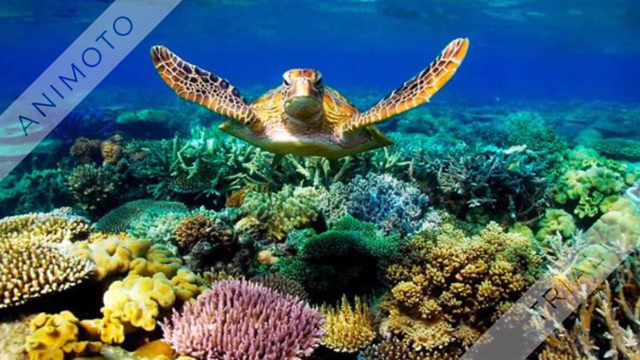 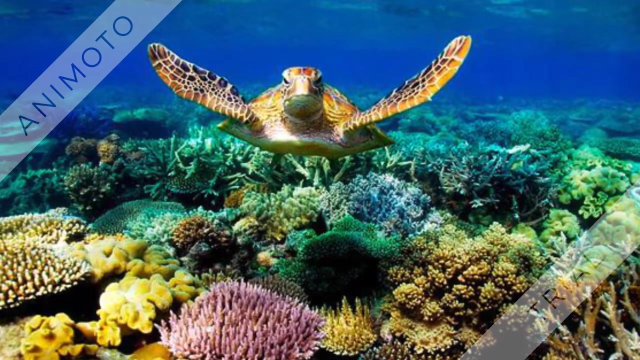 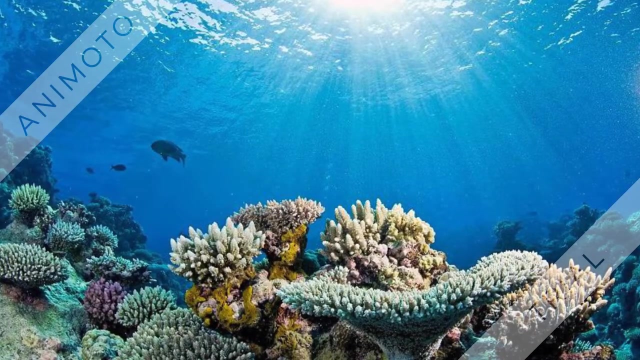 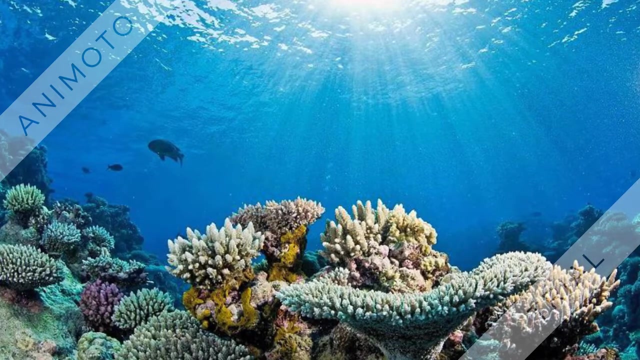 Our oceans are a majestic place full of beautiful marine life and unknown wonder all around. For us, the oceans provide more than just beautiful scenery. It provides tourism to explore this vast underwater world, fishing for both recreational and economic gain and ecological benefits to our beaches and 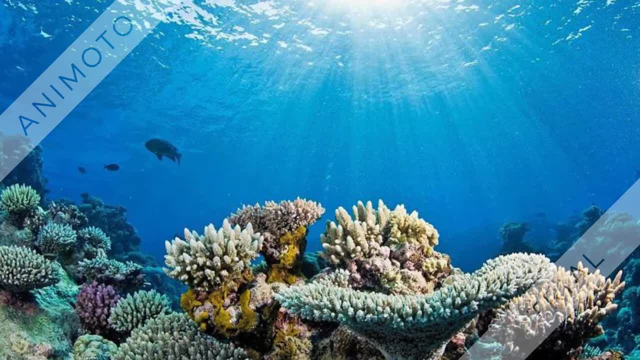 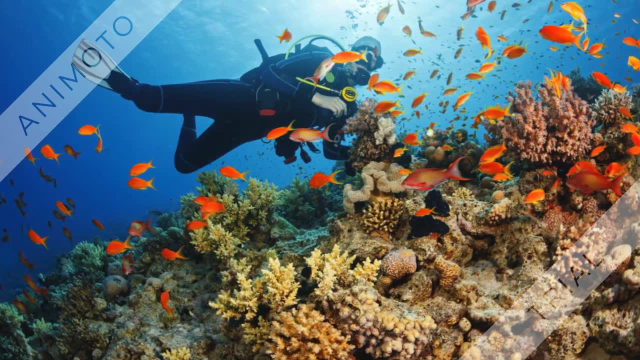 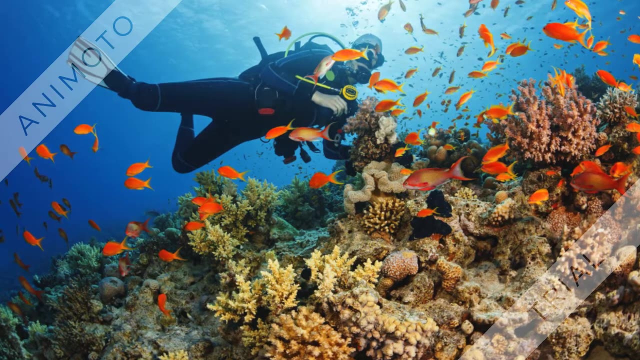 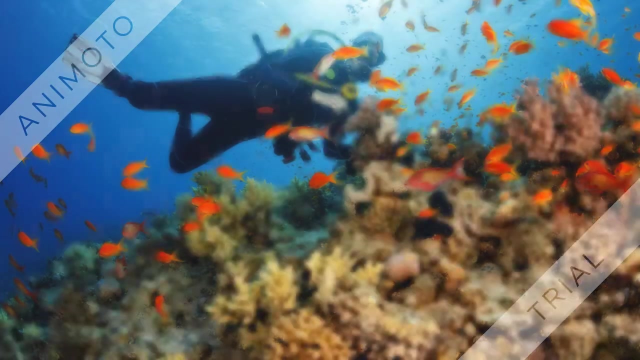 coastal communities all around the world. However, something is happening to our oceans that are degrading them at a rapid pace, and our society and other societies around the globe are contributing to this problem that is endangering the health of our marine ecosystems, A process called ocean. 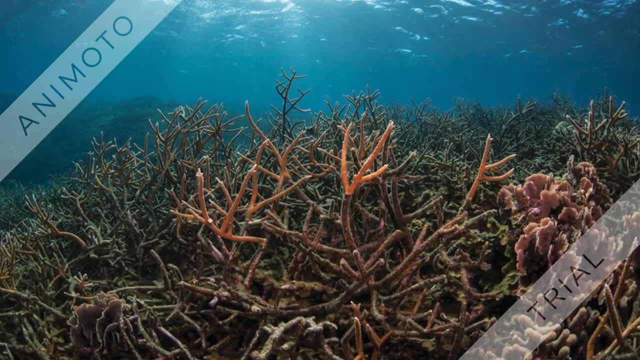 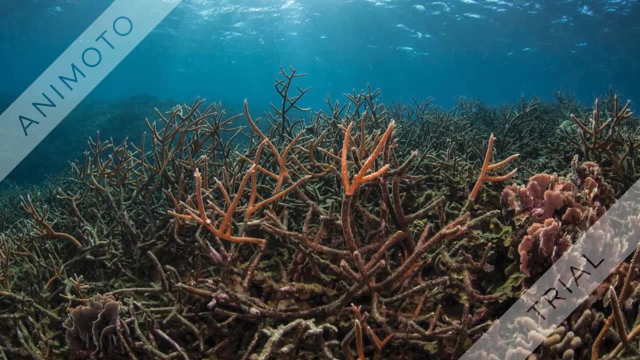 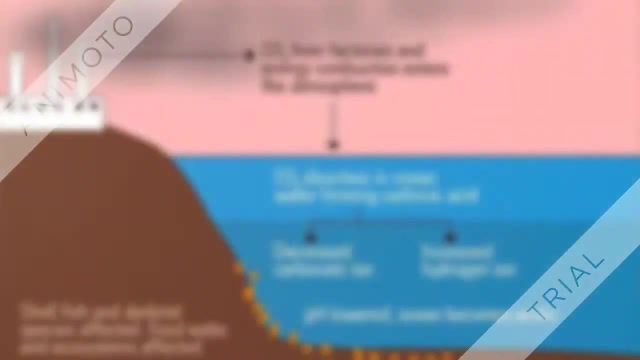 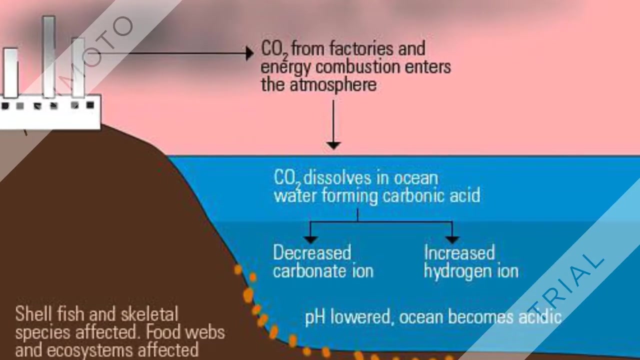 acidification occurs. when carbon dioxide is absorbed by seawater, Chemical reactions occur that reduce seawater pH, carbonate ion concentrations and saturation states of biologically important calcium carbonate minerals. This process has been increasing rapidly and to today, since the Industrial Revolution of the 18th and 19th century, predominantly in America and in Europe. 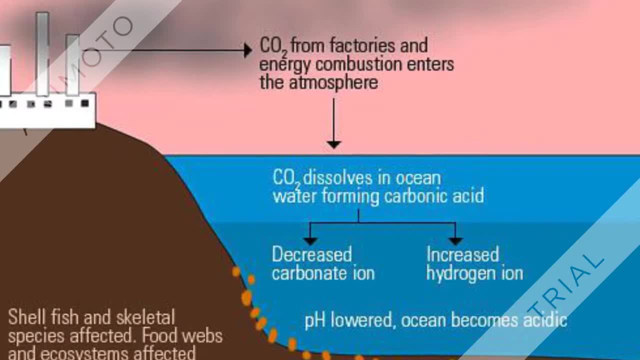 This is when more carbon dioxide has been emitted into the atmosphere by fossil fuels. This has continued, since more countries around the world have been producing more carbon dioxide than ever before. This has continued since more countries around the world have been producing more carbon dioxide than ever before. 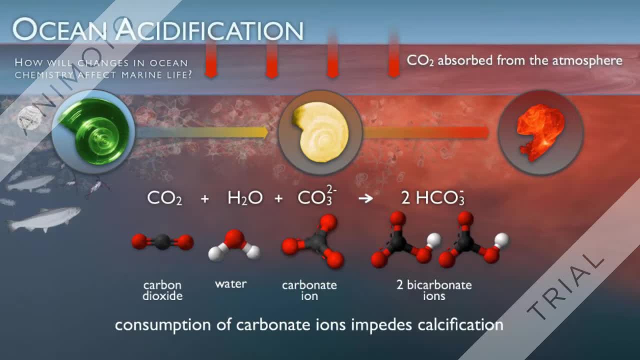 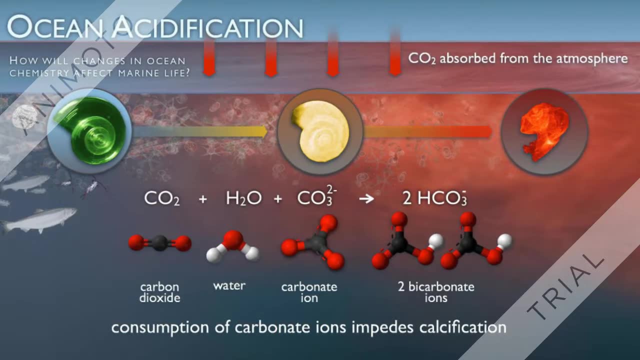 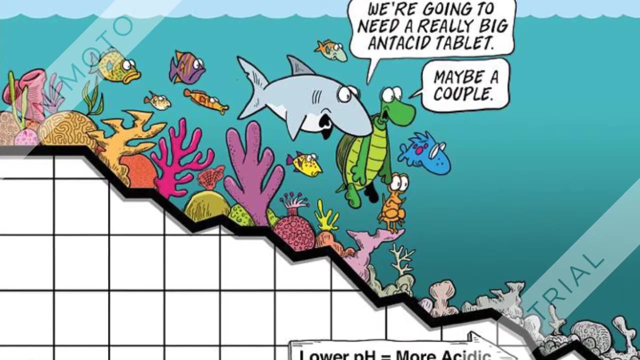 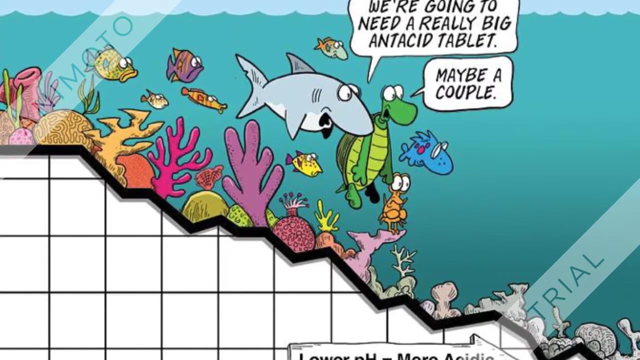 This has continued, since more countries around the world have been producing more carbon dioxide than ever before, Other greenhouse gases into the atmosphere, resulting and more ocean acidification. This is significant because ocean acidification changes the entire chemistry of the ocean, which effects marine animal life, marine 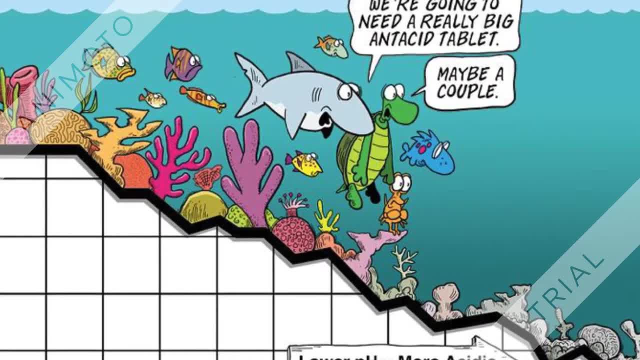 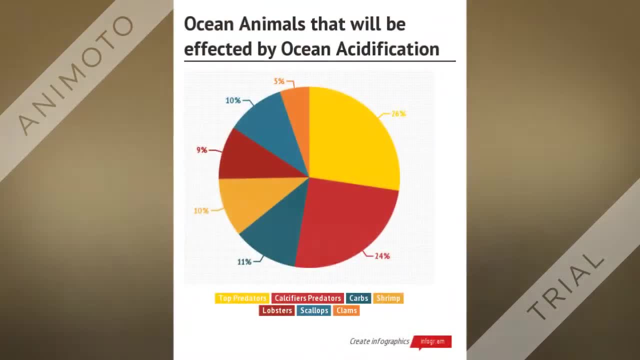 structures like coral reefs and compromises the geochemical environmental commitments of the marine ecosystem. It has been殇цев은 processes of the ocean, which play an important role in local weather and global climate, To the marine life that have shells that are made up of calcium.